I am Anil Kumar. In this video we will understand how to find area of the given figure. The question is: write an algebraic expression to represent area in the figure in simplified form. So that's the figure for you. You can always pause the video. answer the question. 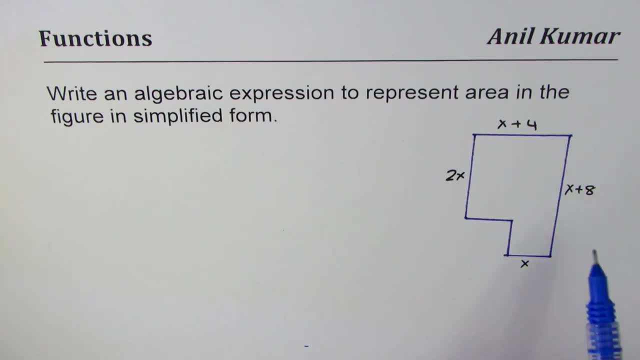 and then look into my suggestions. Now, there are many ways to do it. One way is that you could divide this into two pieces, kind of like this: Find area of these two pieces. Or what you could do is you could divide like this: Find area of these pieces. You could. 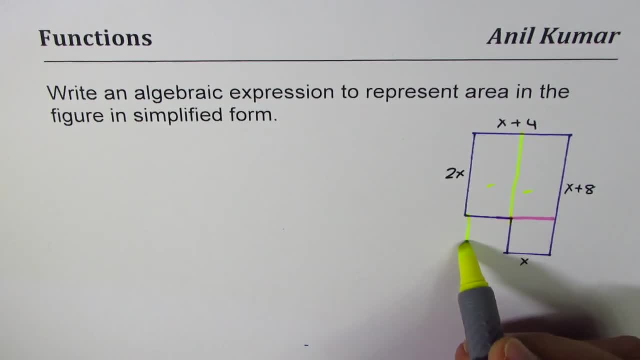 also do one more thing, that is, make the whole block and take away this portion. So definitely, there are three ways, as you can see. So I like you to explore, find the area using three ways And see if you get the same result. 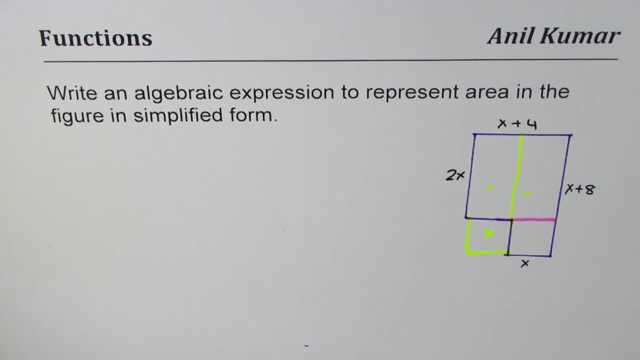 So let's do it. The method which I am going to adopt here is any one of them. of course, We could do any one of them, So let me take this one, So I will do only by one method. So think I have made a division like this, So I have got two areas. This is one, And 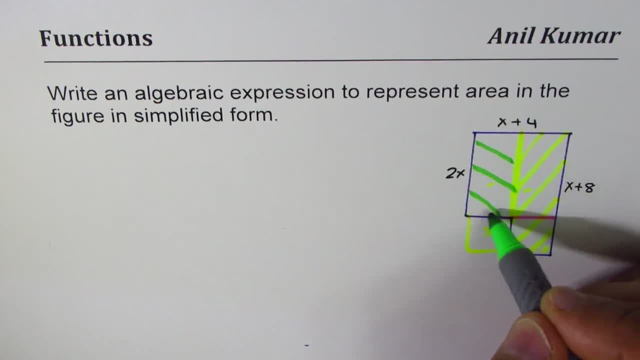 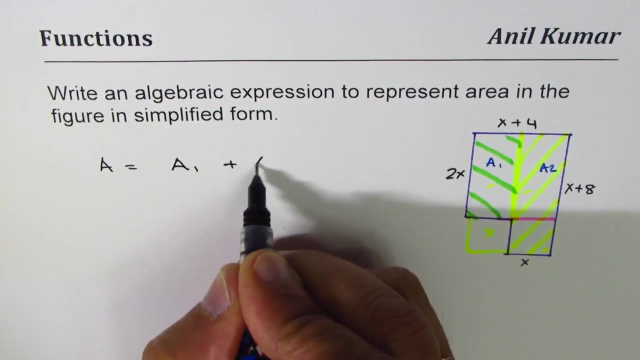 the other one is this one, So I will just add these two areas. So I will add these two areas. Let me call them A1 and A2.. So total area of this figure A will be sum of these two areas, A1 plus A2.. Now what is? 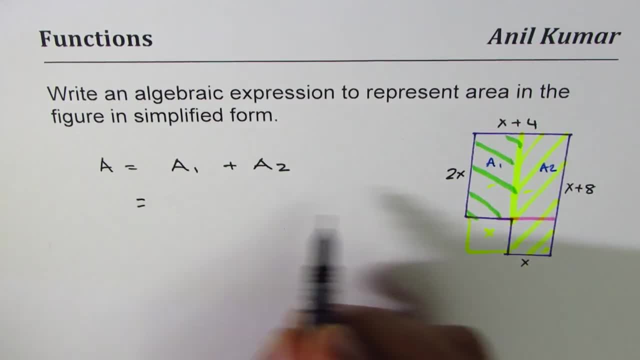 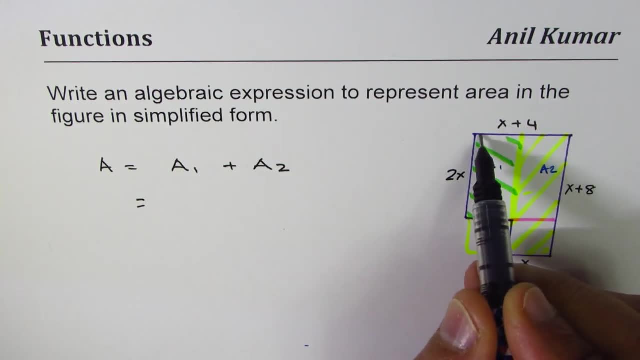 the area of A2? This whole block, And what is the area of A1? This small block? Now, we know this side is 2x. However, we don't know about that side, Since this much is x, this is x. So we know the remaining portion is x plus 4 minus x, So this has to be 4.. Correct. 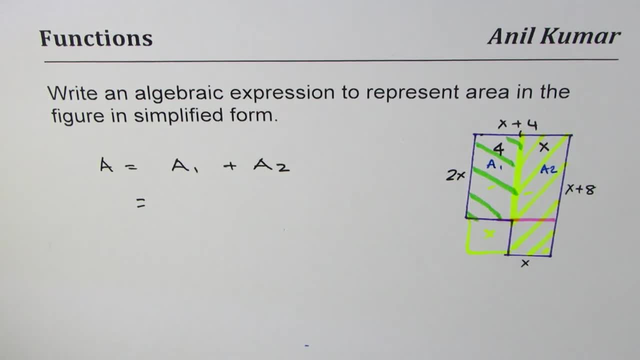 So what we get here is is combination of 4 and x, Correct, So this much is 4.. And that much is x, Is it okay? So it makes x plus 4.. The length is x plus 8 for the yellow portion.